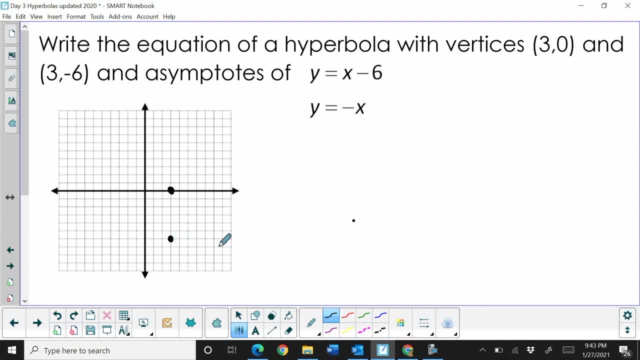 faces. If this is a vertex, it's going to go up and down. So my y squared is first, minus my x squared. I'm still going to have to plug in my center my a's and b's, all that, But I can kind. 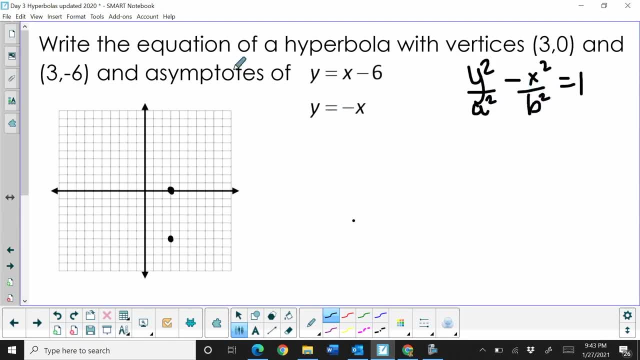 of get a gist of what my equation is going to look like. Now, the next thing we're given is the equations of the lines for the asymptotes, So let's graph each one of these. I'm going to start with this one: y is equal to negative x. Well, that's just got a slope of negative 1.. So I'm 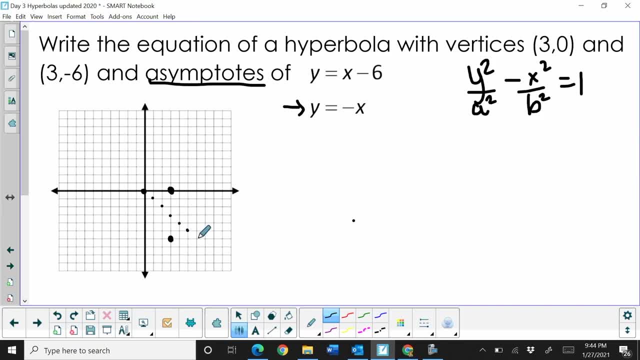 going to dot that in. Okay, so here's the equation of that asymptote: y is equal to negative x, So it's going right there, which looks right, because it's looking like it's hitting this halfway point between my two vertices. So the second one is x minus 6.. So we go. 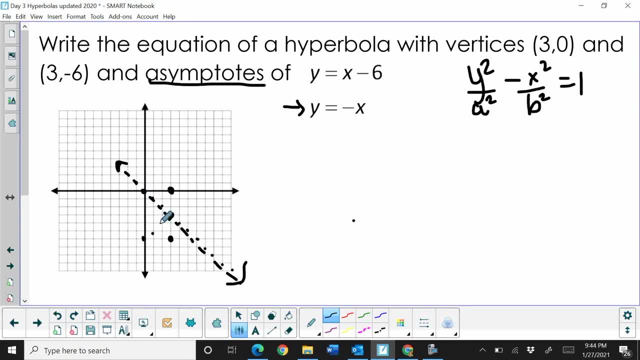 down to our y intercept of negative 6.. And then we go up by 1.. Yes, they're both crossing at that little point. Now let's figure out what that center point is. The center point is 1,, 2,, 3 down. 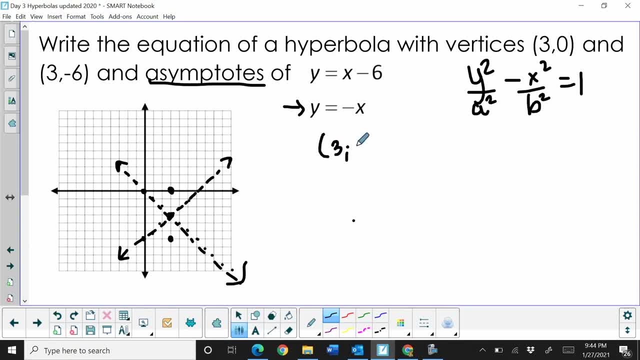 So it is at positive 3, negative 3.. And that is the center of our hyperbola. That's the h and k. we're going to plug into the equation. Now we need to figure out what a and b are. Well, we're going to use the slopes. What is the slope? The slope is 1 and 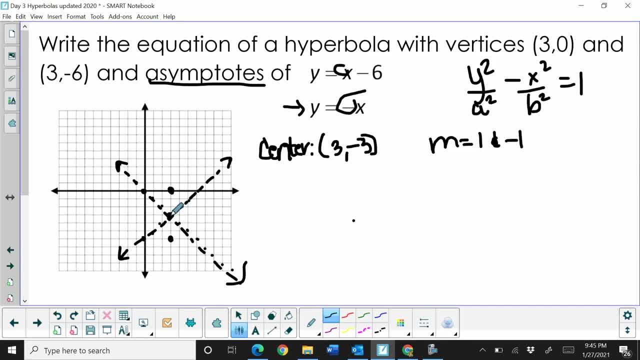 negative: 1.. So, since this is up, 3, if I go over 3, that gives me my box I can draw. So there's my box. So guess what? a is 3, and b is 3.. We haven't had one like that, where a and b are the same, and that's okay. 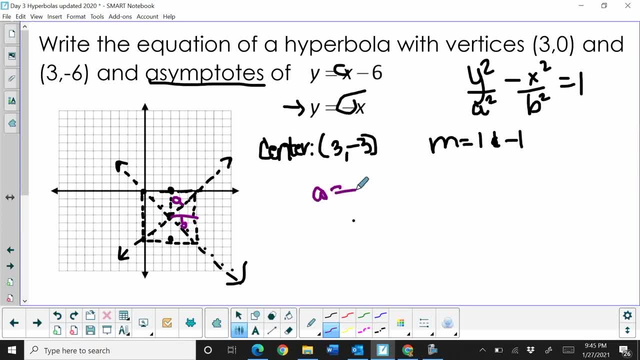 Okay, so a is 3 and b is 3.. So a is 3, b is 3.. And that's all I need to finish out my equation, since I have the center. So let's write our formula with the y squared first.